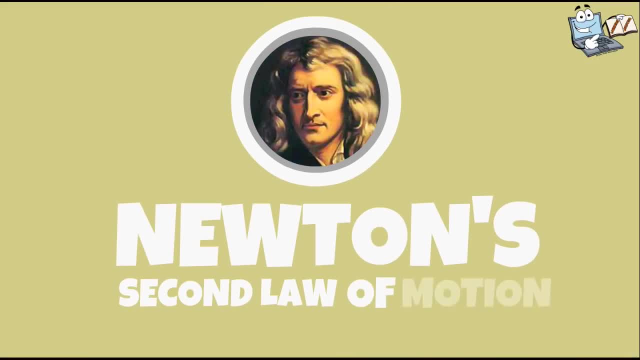 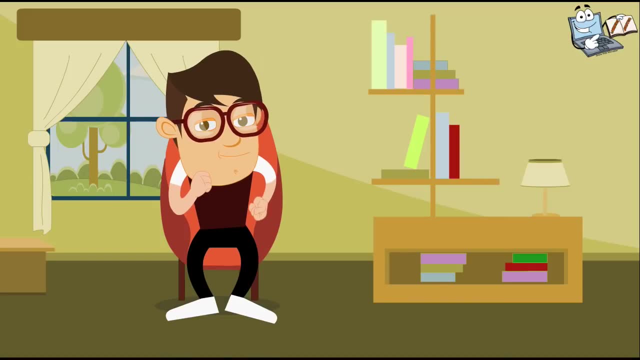 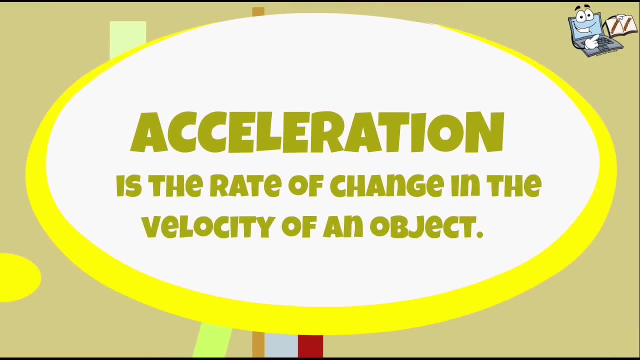 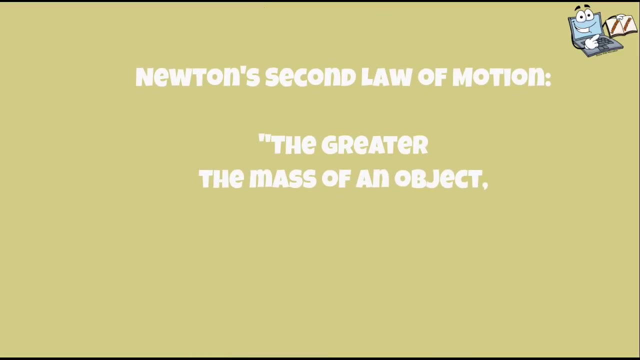 Let's learn Newton's second law of motion. Newton's second law of motion. Before understanding Newton's second law, you must know about acceleration. It is the rate of change in the velocity of an object. The second law of motion states that the greater the mass of an object, the more force it will take to accelerate the object. 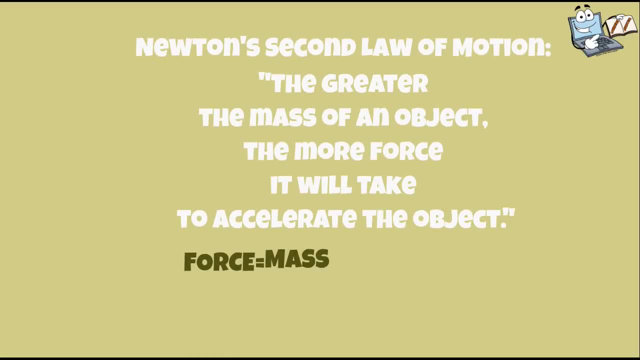 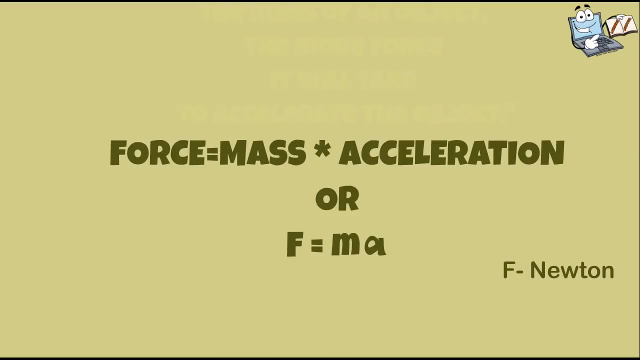 There is an equation: Force equals mass, times, acceleration. or you can say: F equals m into A, Where F is the force and its unit is Newton, m is the mass and has the unit kilogram, and A is the acceleration, which has the unit meters per second squared. 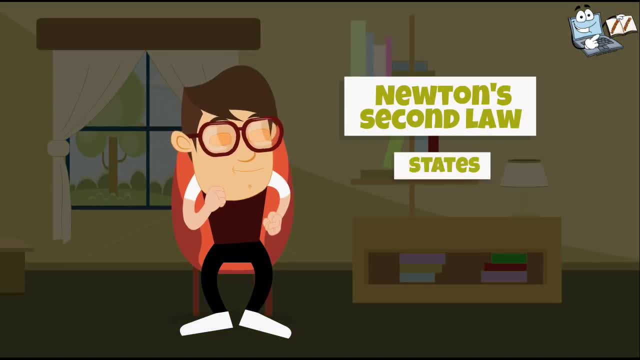 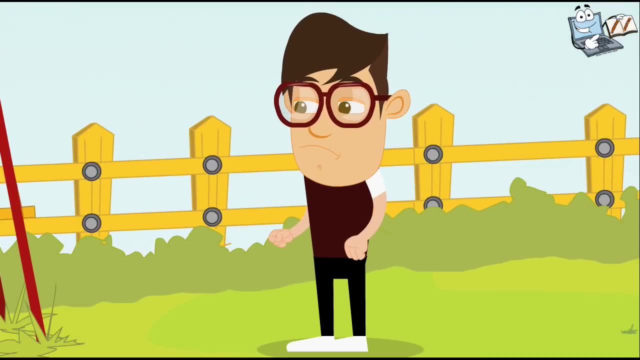 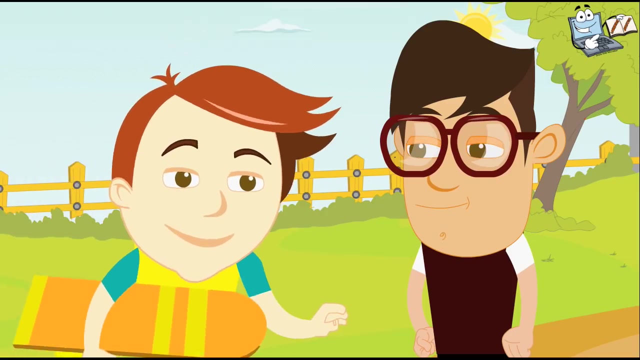 In simple language, Newton's second law states how force, how fast an object can move. This also means that the harder you kick a ball, the farther it will go. Oh, it seems you are not understanding this. Your friend is on a skateboard. 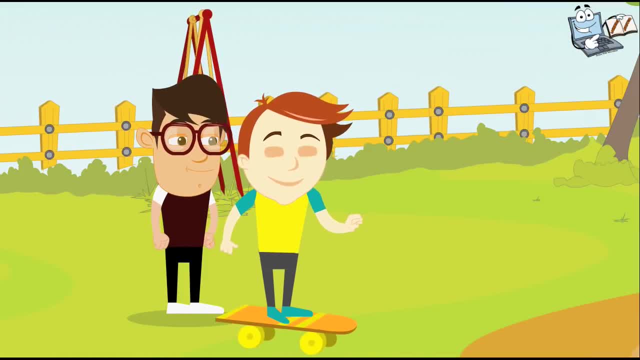 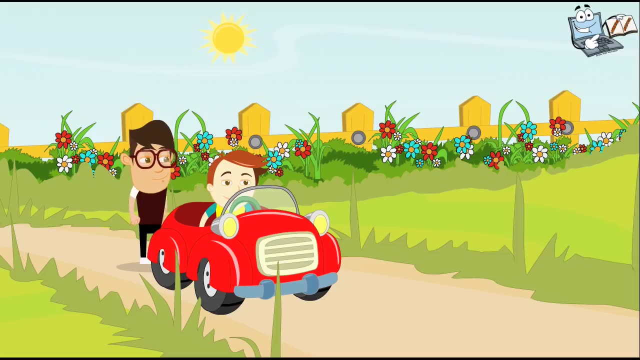 You push him forward and he begins to move slowly. Now a big push and see, much faster. Now your friend gets in his car. You push the car, but it is so hard to move. You pushed harder and it barely begins to move. 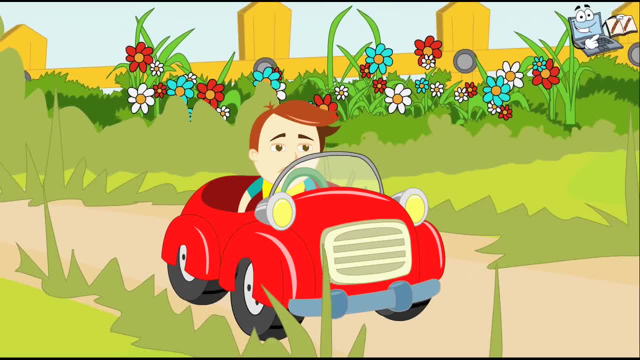 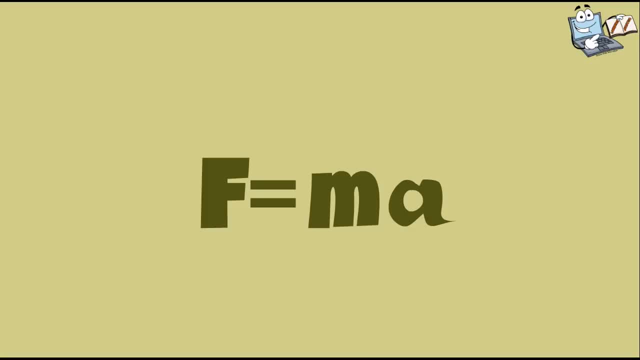 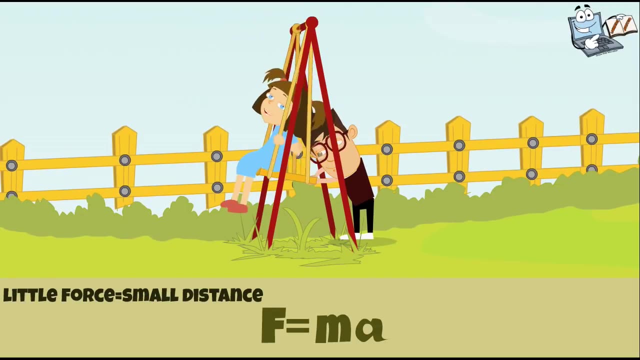 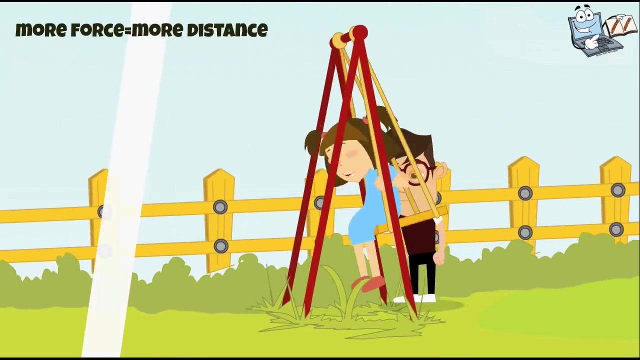 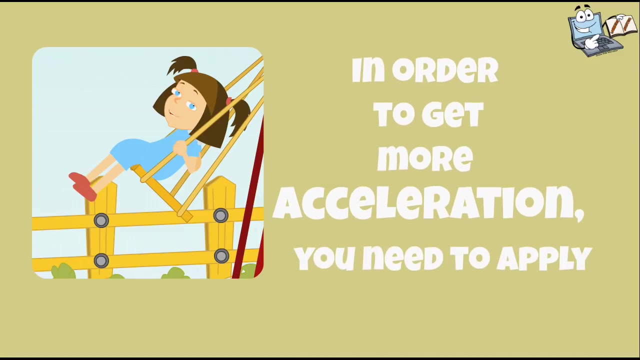 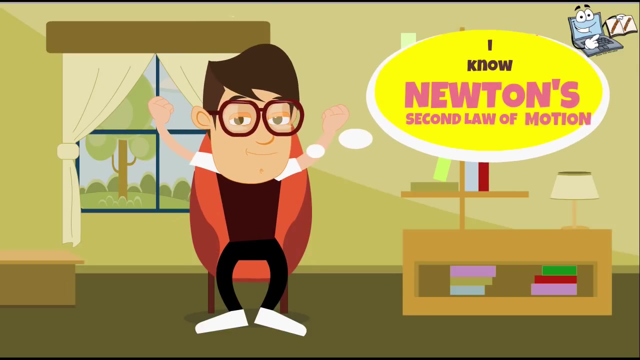 Oh, and now you are pushing it with some other friends. See it moves faster and faster. Move it so fast because you are a guys. Show them, The harness is lagging so hard because there is no acceleration. you,